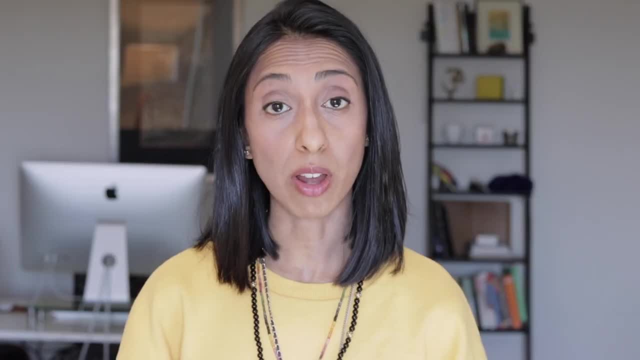 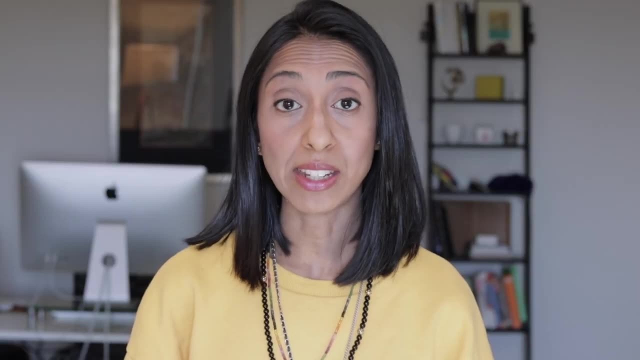 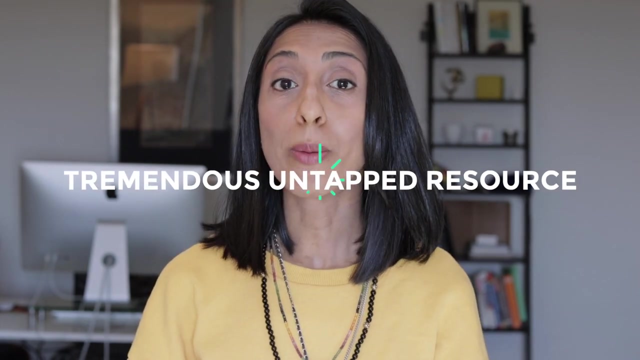 as a committee to take inventory of their current digital product design assets. They come to a consensus about what else they might need and how things ought to be designed, presented, coded and talked about. But beyond creating and implementing a design system for yourself, design systems are a tremendous 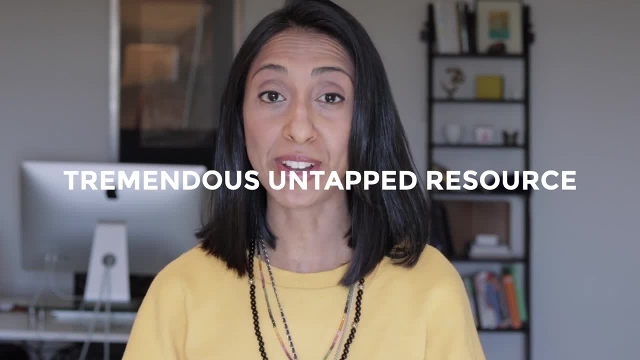 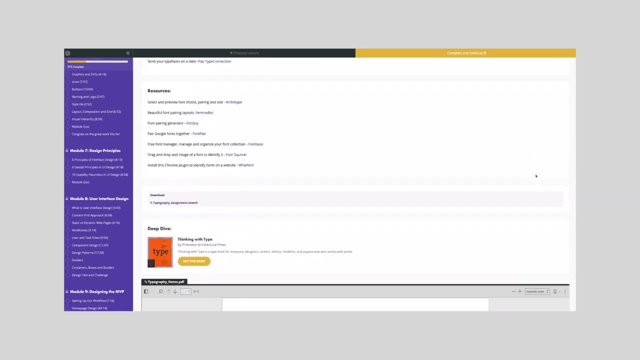 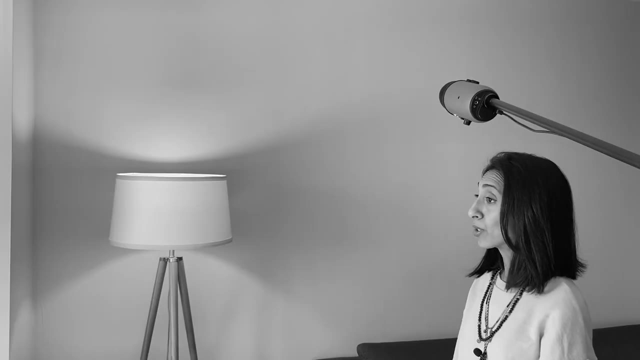 untapped resource for learning how to create better user experiences and interfaces just by studying them. At DesignerUp, we've been framing design systems as a teaching tool with our product design students to help them better understand, explore and learn the best practices and principles of UI UX. 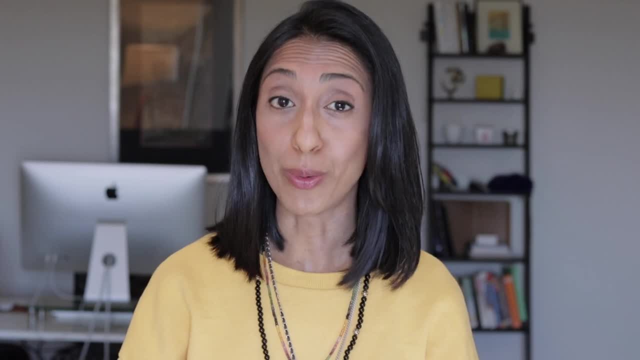 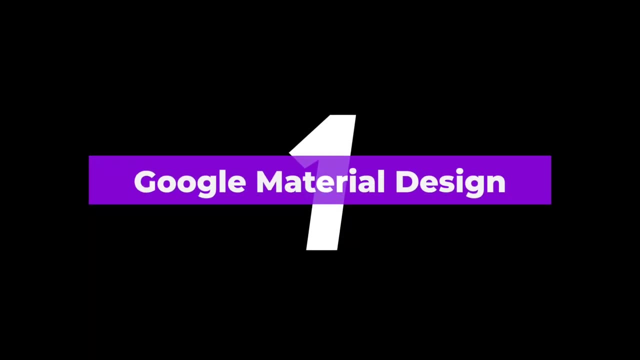 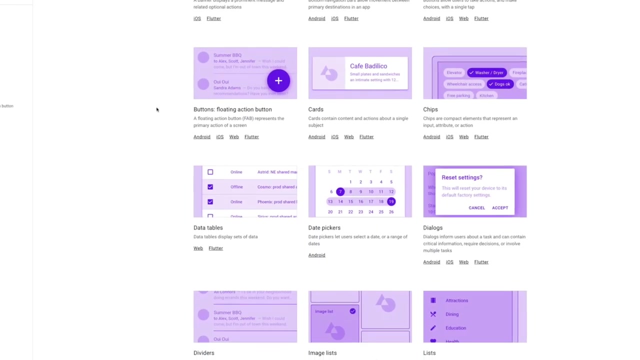 and product design from some of the best companies in the world. Here are five of our top favorite design systems and how you can learn from them. Number one: Google Materials. Google's publicly shared material design system paved the way for many to follow. Google categorized and cataloged components in a way the design world had. 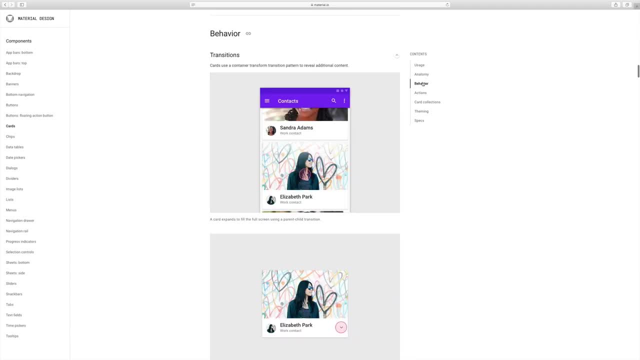 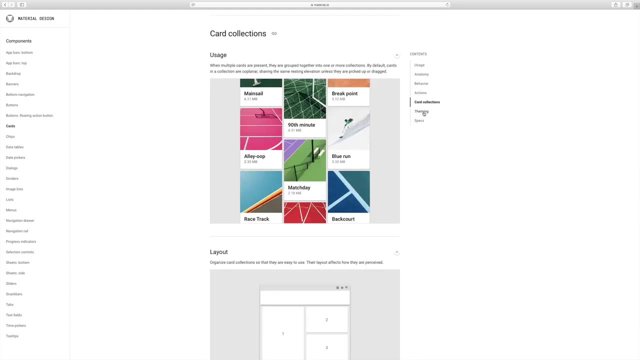 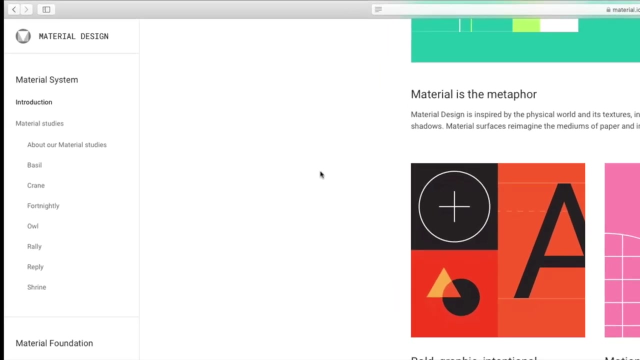 never so succinctly seen before. They made the mistakes so you don't have to- and gave order and meaning to the atomic design principles that all design systems are built on. today They call it material design because it's meant to be a metaphor inspired by physical world, textures and actual material. 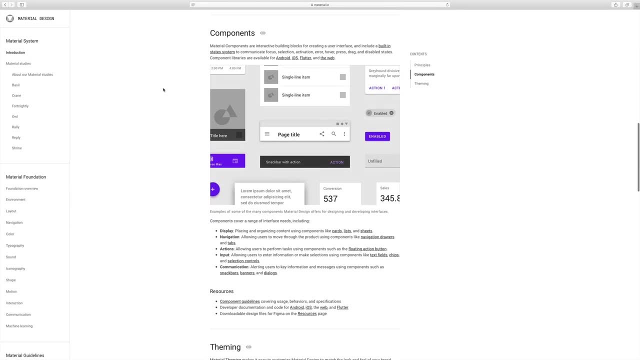 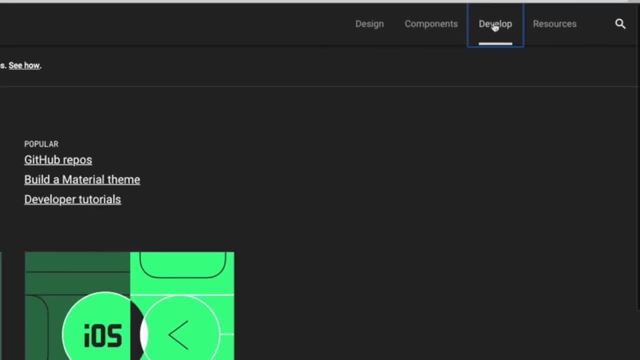 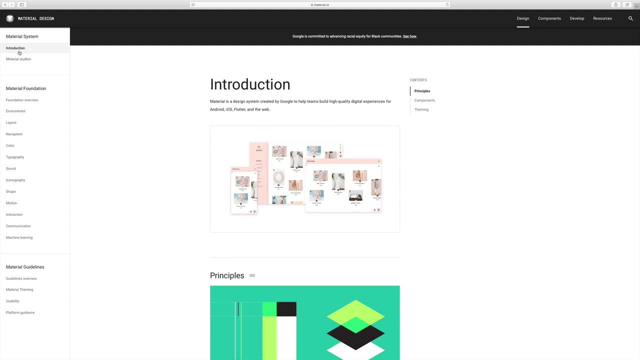 How light reflects and casts shadows, et cetera. Material design has four main areas- design components, develop and other resources. If we look at design, we have the material system here, which shows you an introduction to the principles and components: theming, typography and everything that makes. 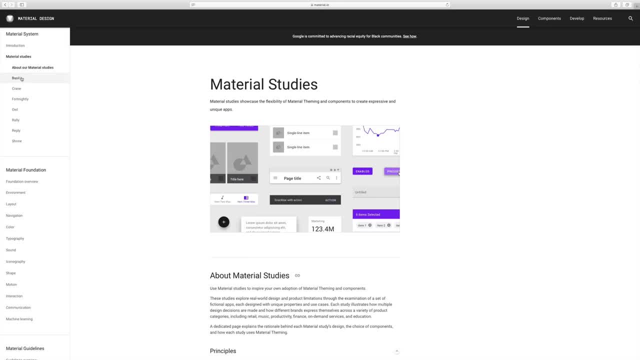 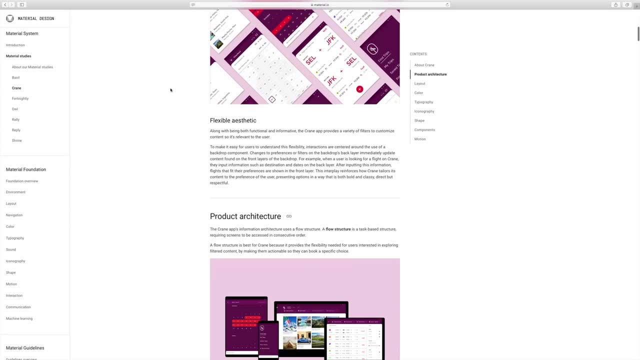 their system. Material studies show the different styles that they use for their systems. There's Bazel, which is recipe app. Crane, which is great for travel apps. Fortnightly, perfect for news topics. Owl, which is great for educational content. 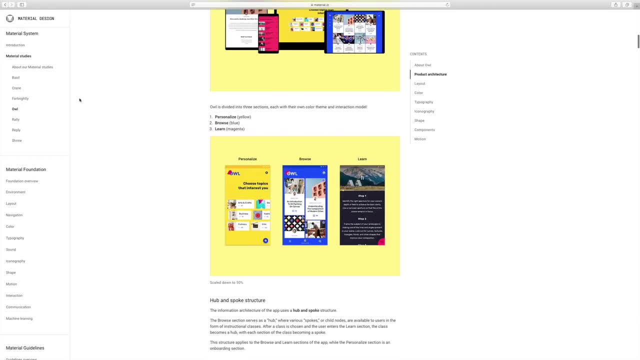 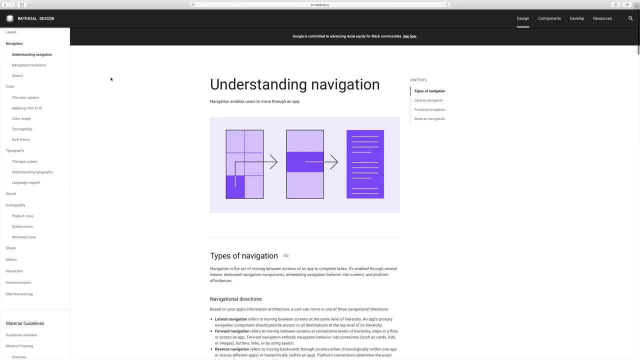 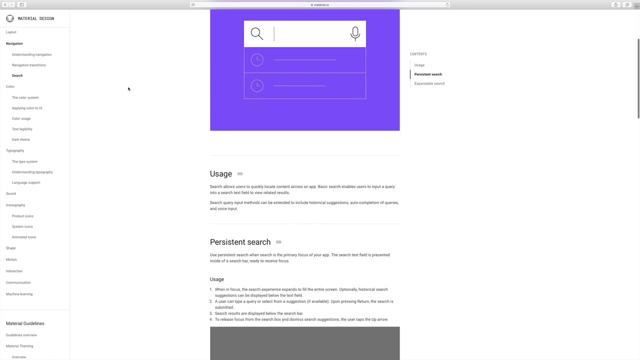 So, as you can see, they've categorized this based on the branding, the color schemes, the typography, and labeled it for different industries and styles of design. Drilling down deeper, you can look at their navigation transitions for navigation Search patterns. 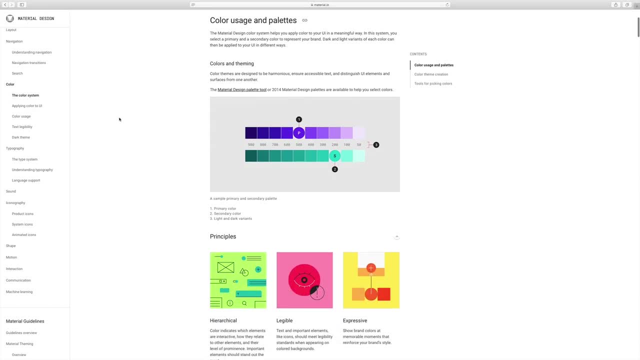 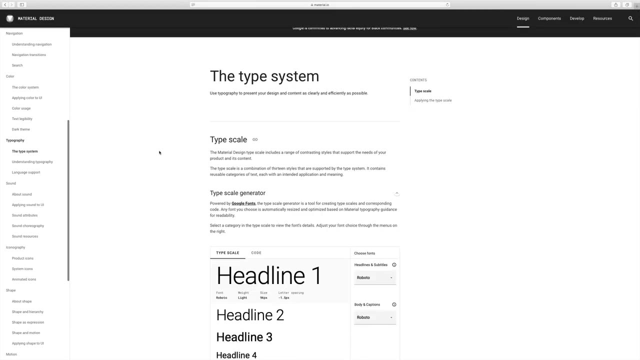 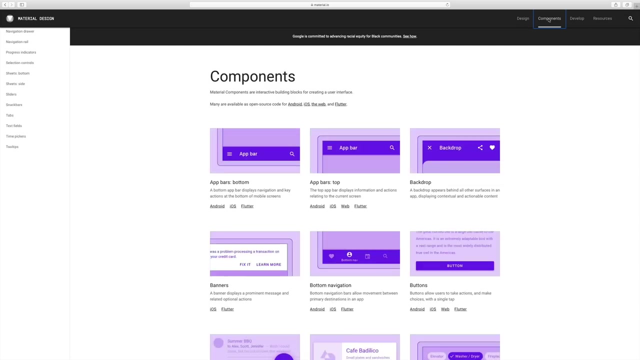 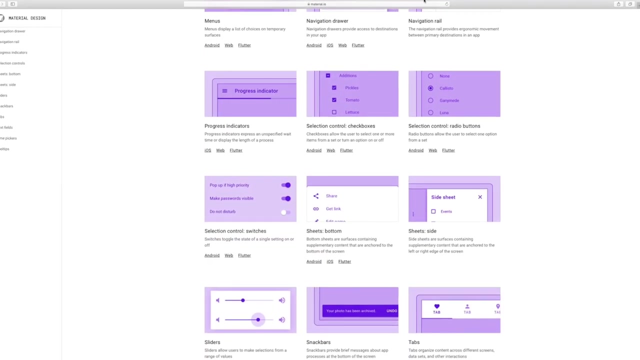 And then moving into their color systems, applying color to UI, dark theming, And the list goes on with typography, sound iconography. Scrolling back up to the top, we get to dive into the actual components. This is such a valuable section because we all use these as universal patterns. 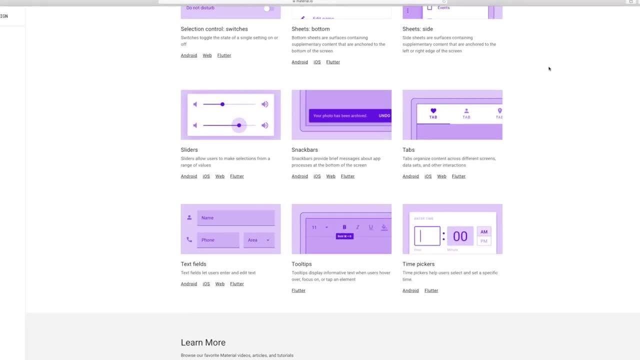 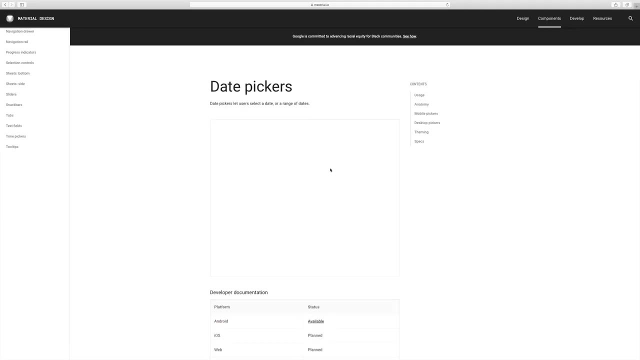 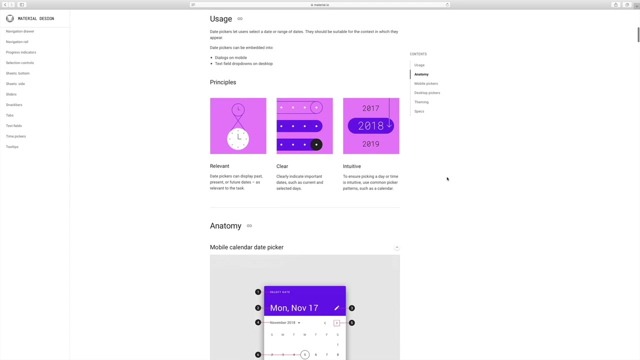 in our UI designs. So if you are just starting a project or a design and you need to design a date picker, for example, what better way to understand best practices and principles for date pickers than looking to Google themselves? So you can see, it's basically like a course in UI and UX design. 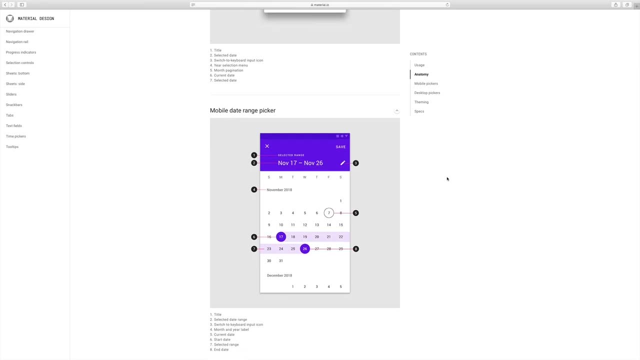 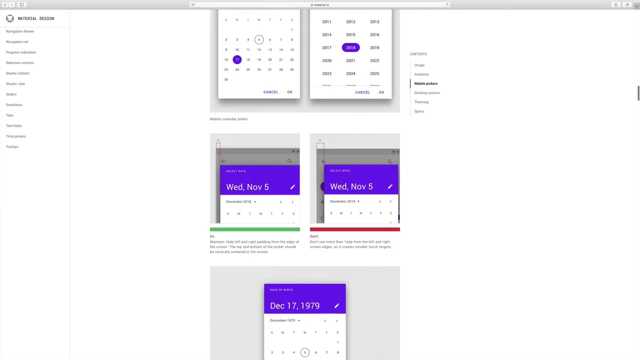 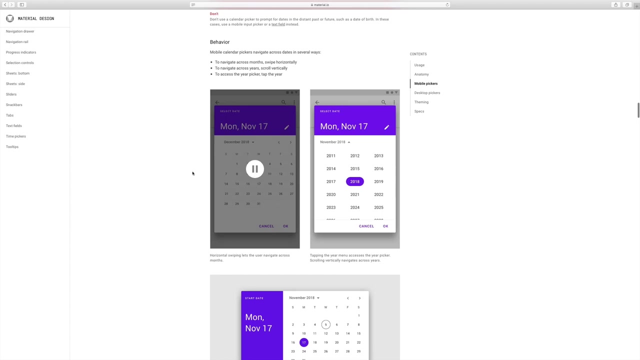 You can go into the principles behind why the date picker is designed, the way that it is, the actual anatomy And the parts and elements and components that should be in a good date picker, And you can also understand behavior by looking at their animations and micro-interactions. 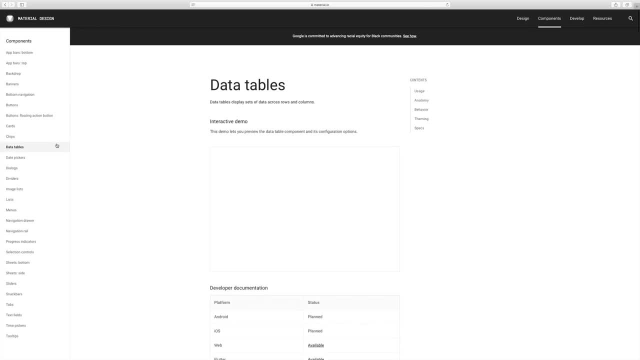 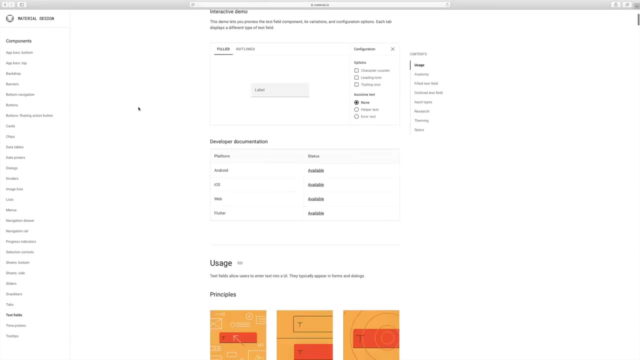 And you can do this for every single component and element you can think of, Whether you're having trouble organizing a lot of data into data tables or you're making a menu or sub-menu or navigation. it's all here, From tabs and text fields. 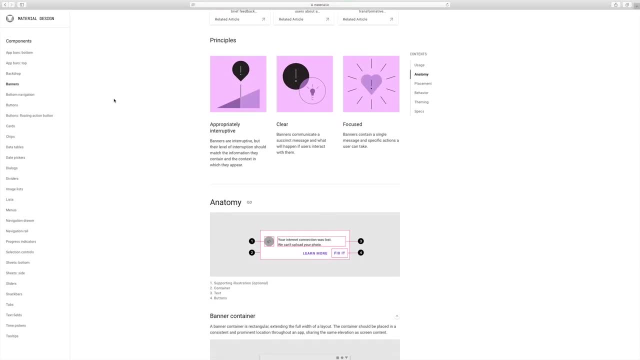 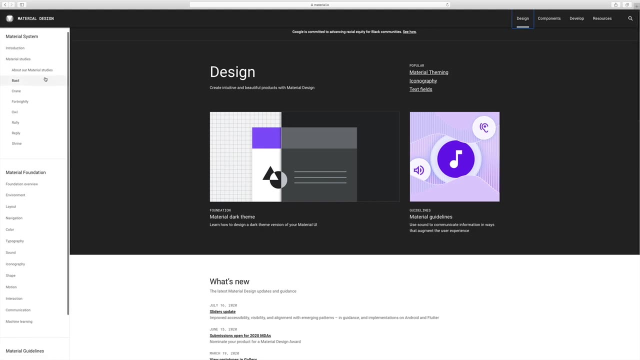 to tooltips and banners. Everything you need to know- that's been tested by Google themselves- is in here. So one way to use this is to go back to the design section And let's say you're designing a retail, e-commerce or fashion app. 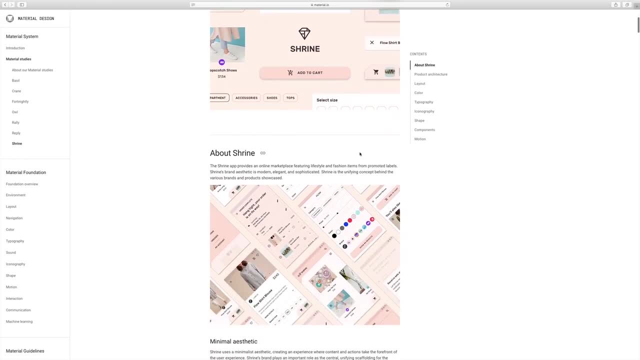 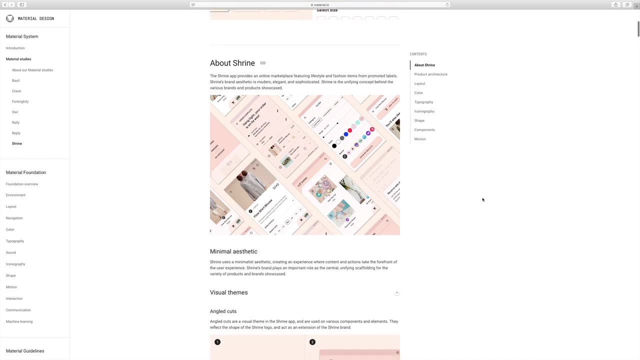 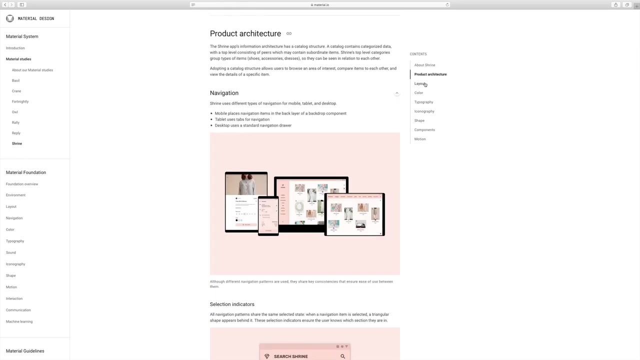 Check out Shrine And you can get an idea here about how they brand and layout and create all the components that go into creating a retail app. So this is great if you're trying to design a shopping cart system, a checkout system and you're in that industry of lifestyle, of fashion. 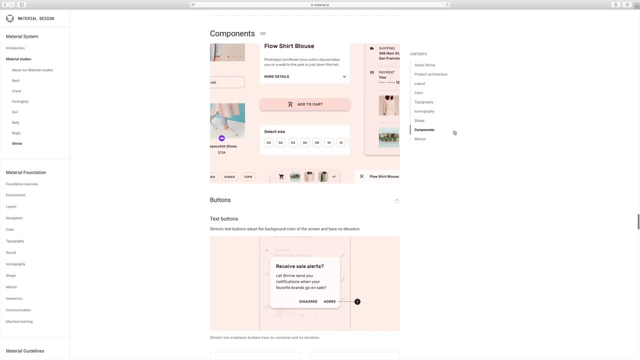 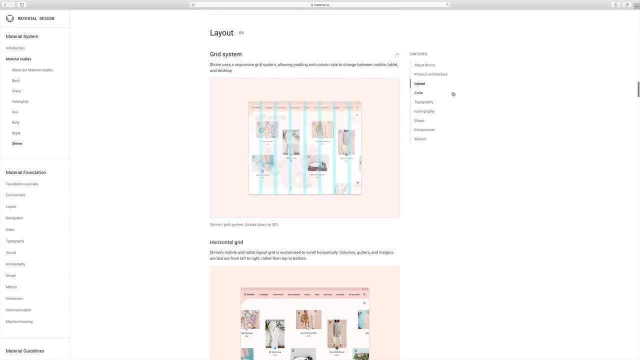 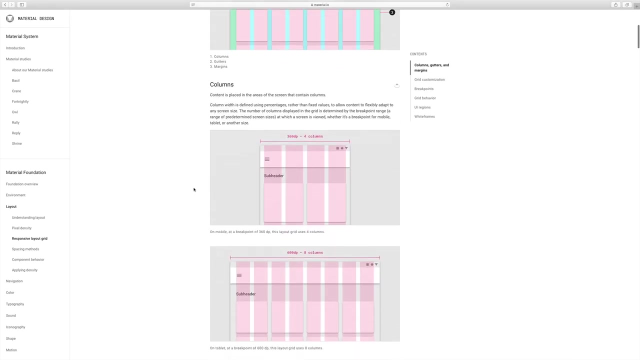 You're not only getting amazing examples of design patterns, but you're understanding the user experience behind it, the intention behind it and the interactions. This is an amazing explanation of the grid system that's being used. So if you're trying to understand responsive design- padding, column sizes, gutters- this 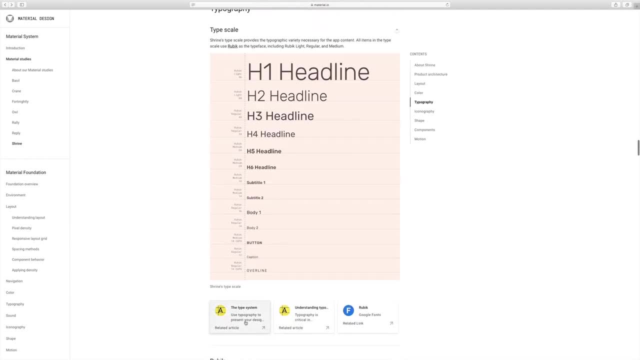 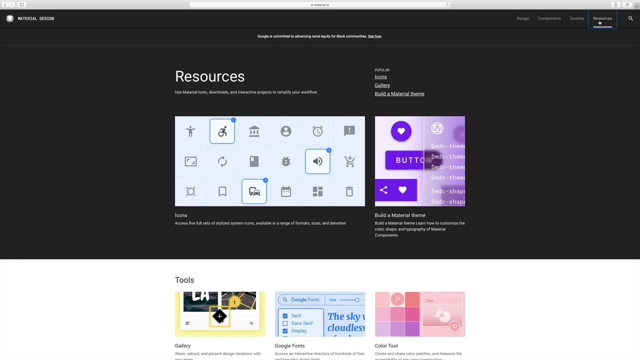 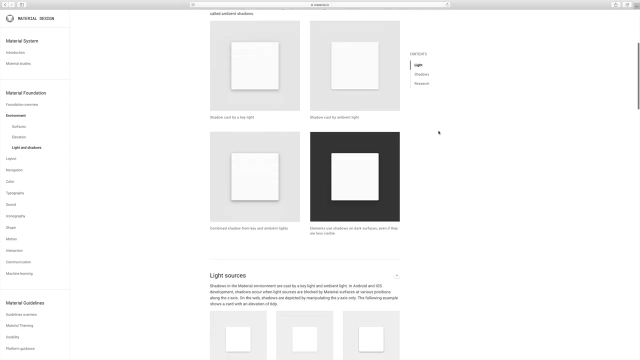 is a great study. You can learn so much about typography scale- the size that your headline should be versus the size of your body text- And if that's not cool enough, you can download these actual resources and design source files on the resources page. 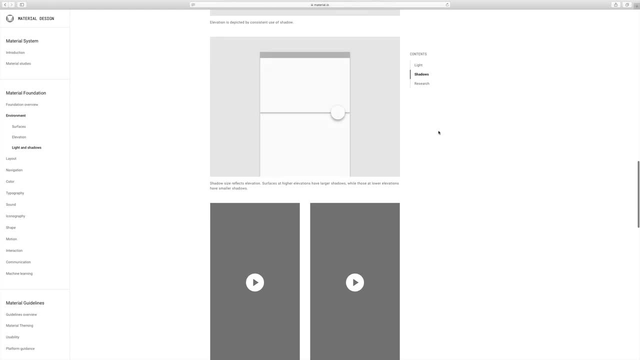 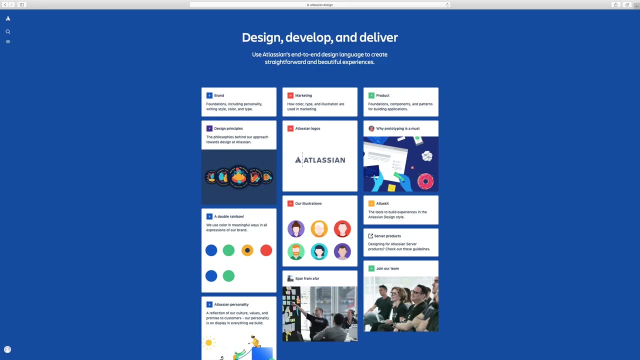 This design system is a powerful learning tool and study, So I highly recommend you check out Material Design. Number two, Atlassian Design System, One of my personal favorite design systems. Atlassian makes project management and collaboration tools like Jira and Trello. 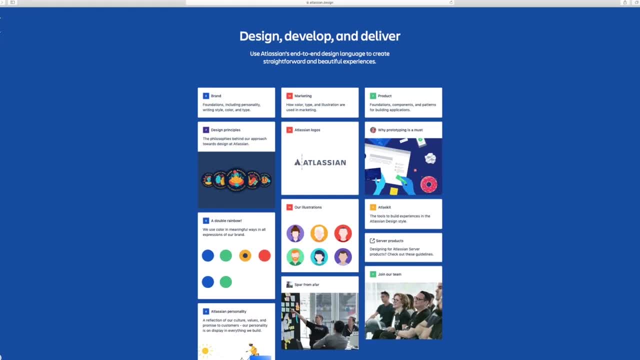 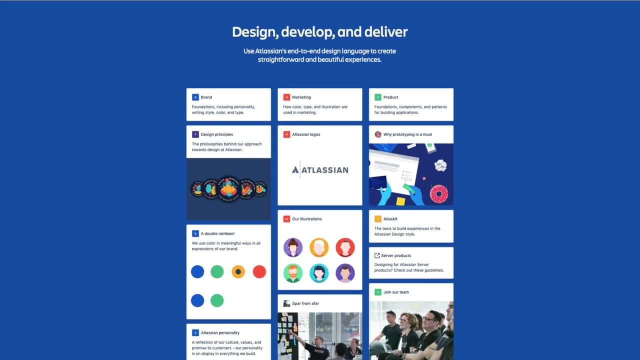 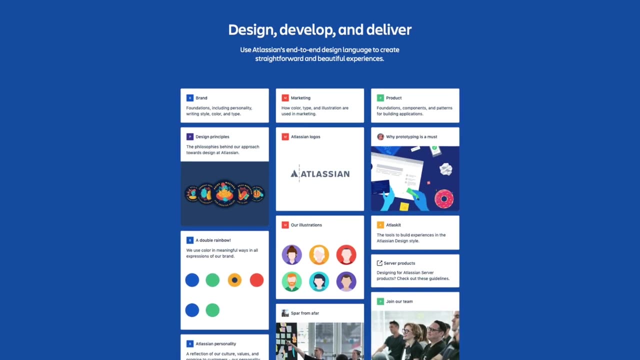 While not quite as big and intricate as Google's material design, you can learn a lot about brand guidelines, design principles and how to design products that are in the collaboration and project management space. So, as you can see, most of the design systems are laid out in a pretty similar fashion. 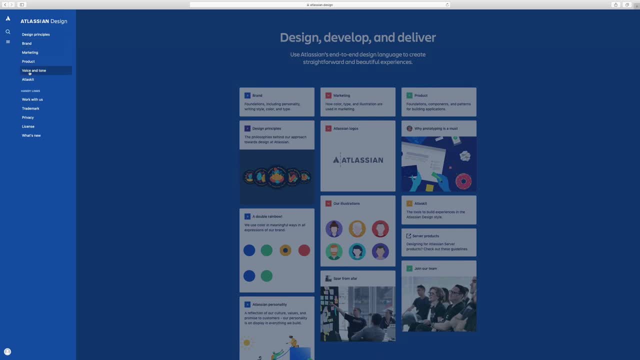 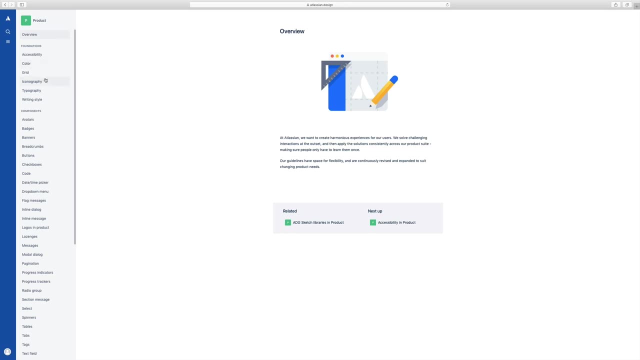 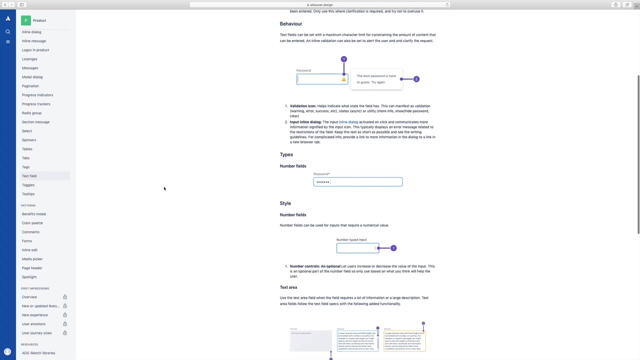 Kind of like a knowledge base That groups things in Into categories. So if we take a look at product, this is where you'll get to see more of the components and foundations And, just like Google Design, you can drill down into how they design text fields, toggles. 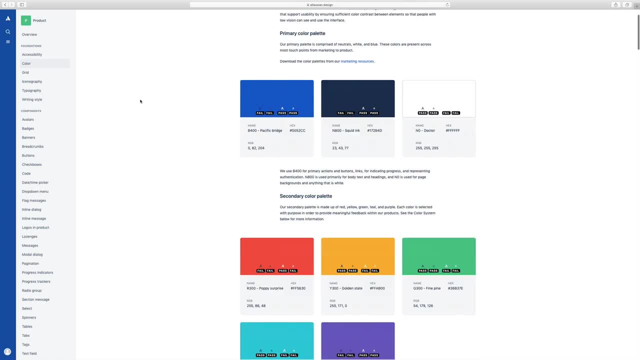 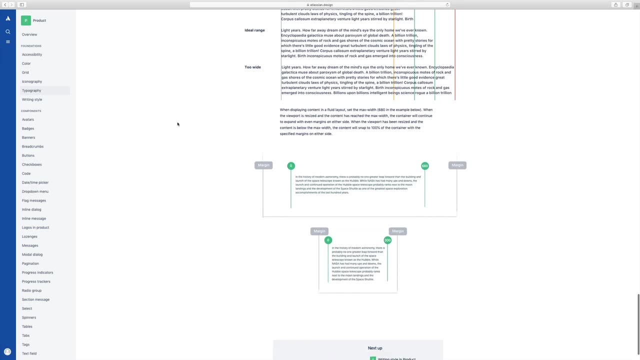 tooltips. I'm a big fan of their style and the color palettes that they use and their typography, So this is another one for you to dive into, to get inspired by And understand How to create project management software Number 3.. 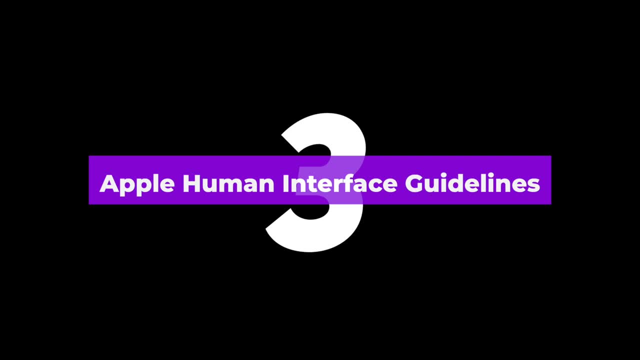 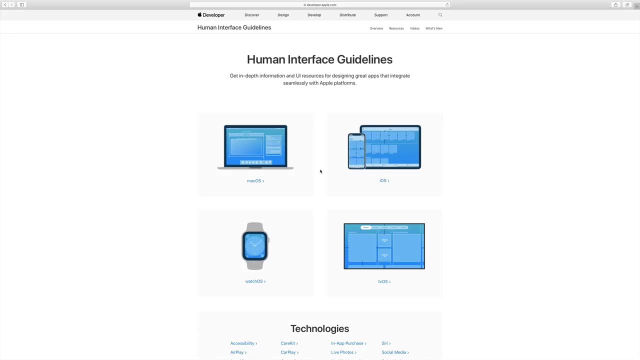 Apple's Human Interface Guidelines. Another massive design system is Apple's Human Interface Guidelines. These guidelines allow you to take a closer look at operating systems including Mac OS and iOS And, going into this, you'll see a lot of the same components and visual design guidelines. 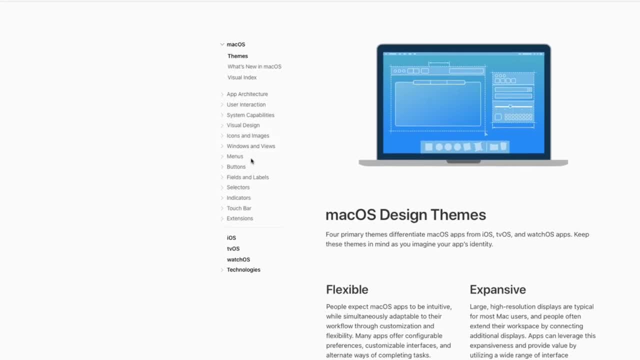 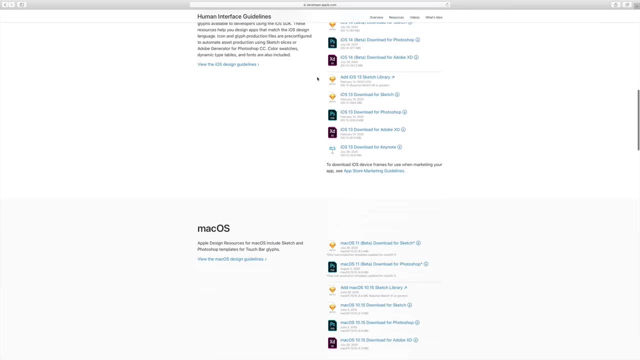 And I think where Apple really excels here is in their resources: Lots of things to download, lots of things to use, lots of things to use in your computer- And I think that's where Apple really excels- To download lots of different source files for various design apps and software. 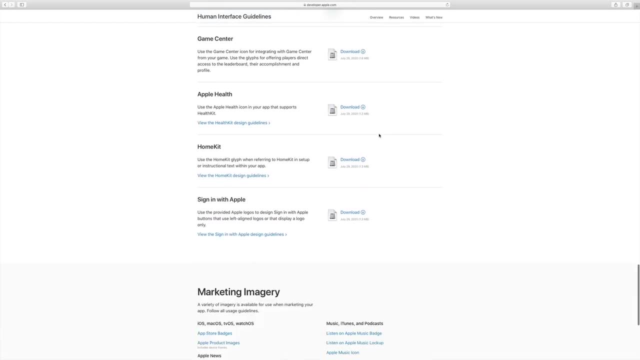 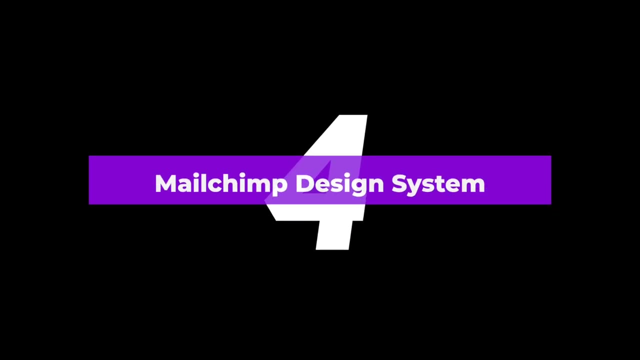 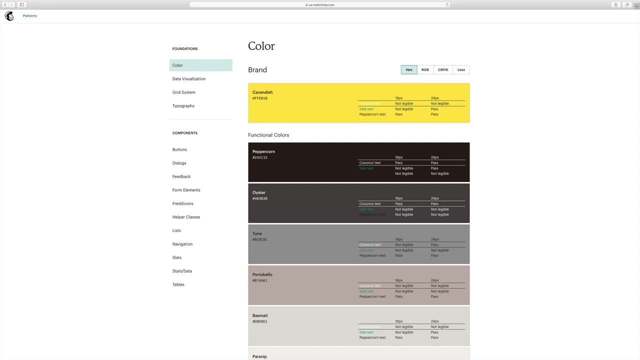 So this is a great one to explore and to look at different devices, smart home things and operating systems. Number 4. Mailchimp Design System. Mailchimp is another great one to reference. if you're working on a project in the realm of email marketing- business ads, Mailchimp can provide some really useful tips and examples. 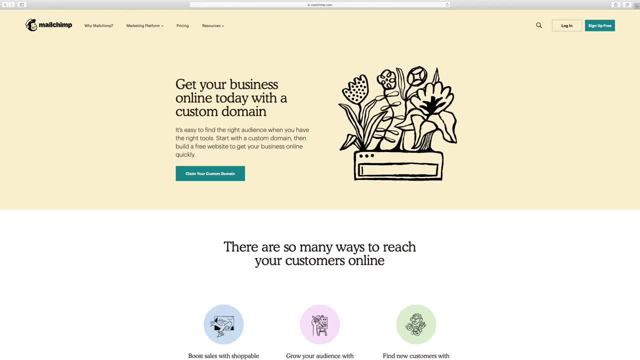 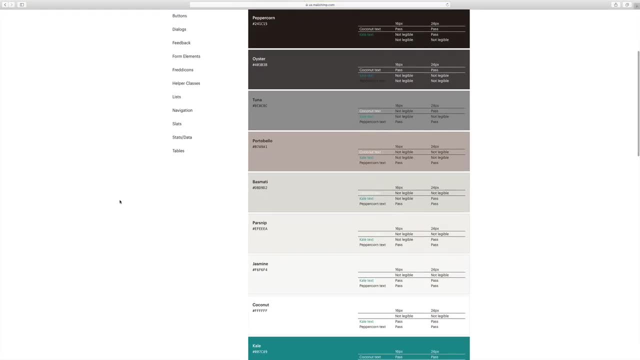 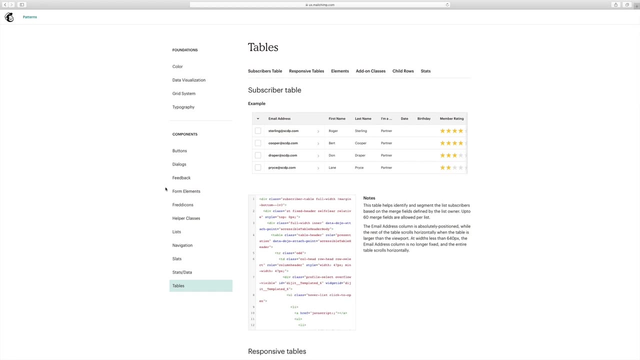 of how to have great UX while still pushing the boundaries of expression and creativity. There are a lot of innovative design ideas to pull from here and ways to make complex tasks and data visualizations a lot more digestible and accessible through approachable and intuitive UX. 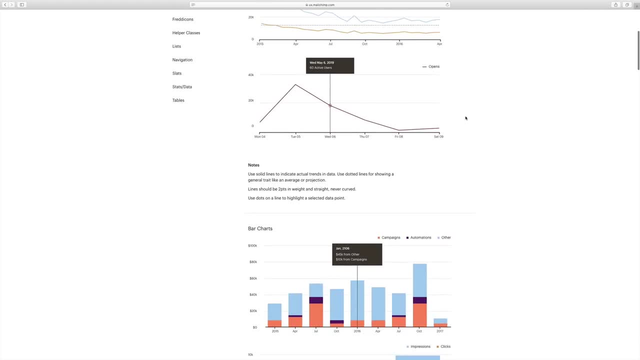 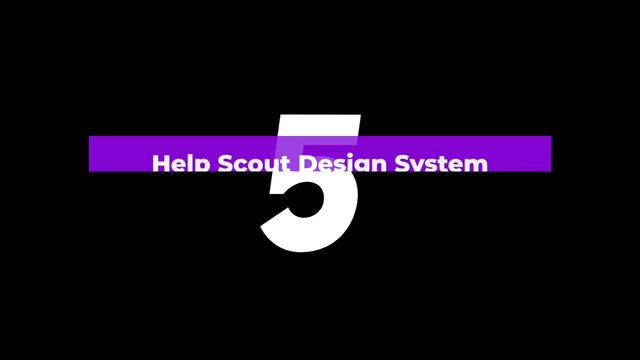 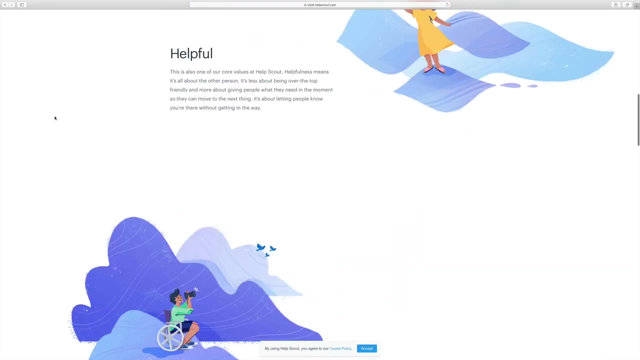 So check this out if you're having trouble designing charts or other data visualizations. it's a really great reference. And finally, Number 5. Help Scout Design System. Help Scout system is much smaller and compact than the other ones we've looked at, but I 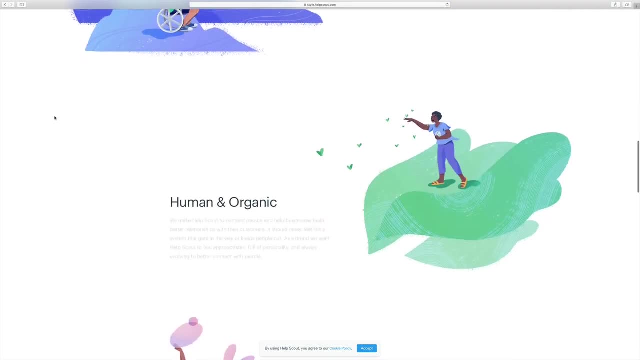 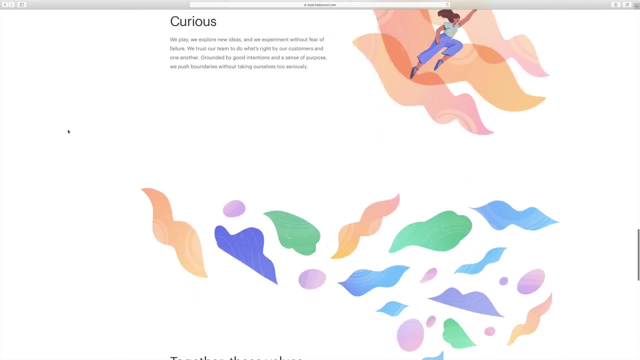 wanted to leave you with an example of something that you can create on your own. Maybe you're starting your own design system, or you're just a team of one or two. This is a great way to start thinking about your own components, your values and your. 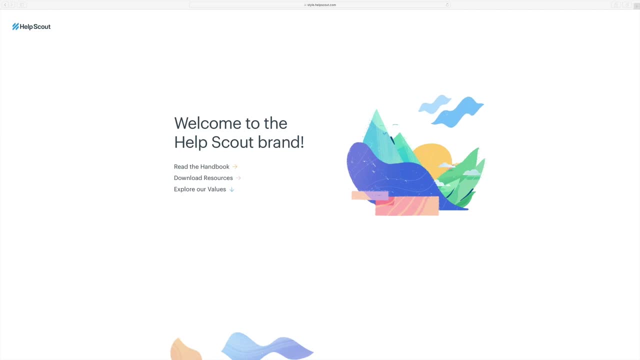 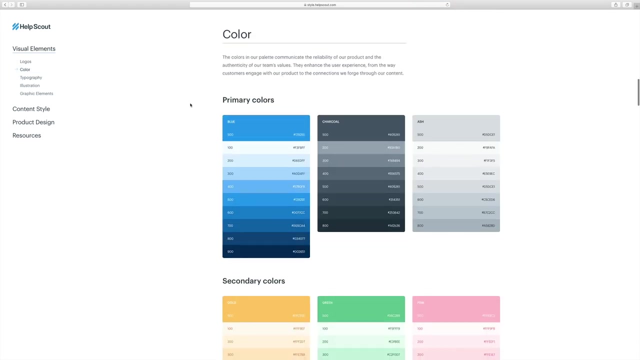 brand guidelines. Help Scout is an online support ticketing system and it's a help desk with a really seamless customer experience. Here you can explore their design handbook and get an idea of colors, logos, typography- I particularly like their color spectrums and color systems- and you can also look more. 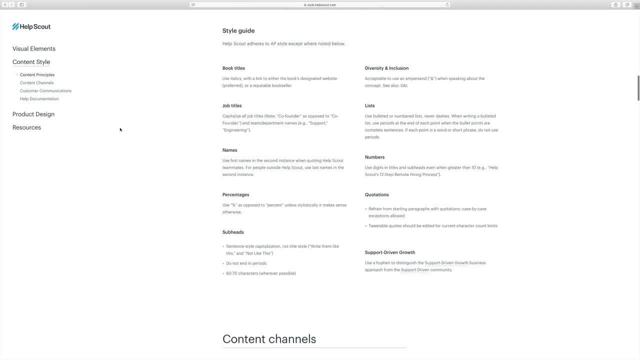 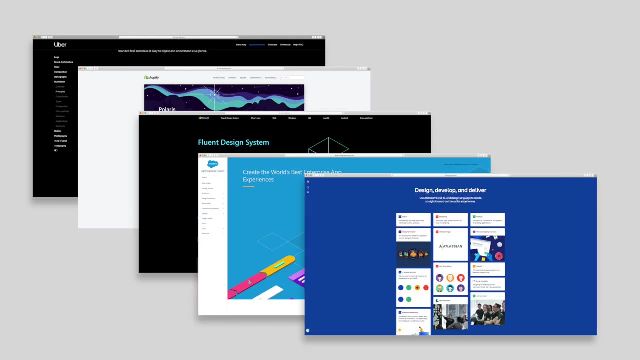 into their content, principles, imagery, language, style, guides, etc. So those are five really great design systems that you can explore, learn from and copy and steal, And there are a lot more in the article on our blog, So head over there and check it out. It's a great resource. I really hope you guys find it useful. Thank you for watching and I'll see you next time. Bye. 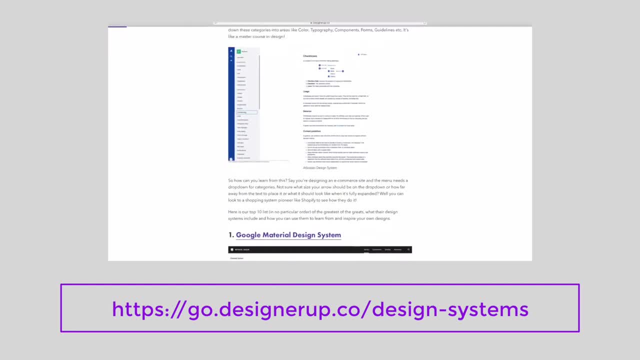 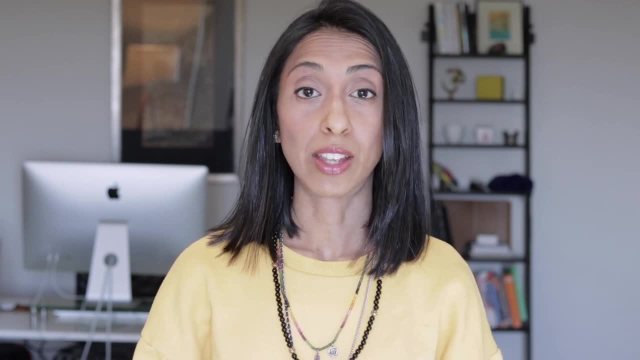 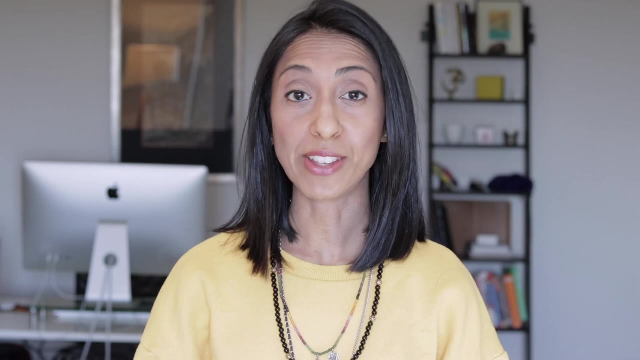 over to designerupco slash blog to explore more design systems. Believe it or not, there's even more to product design than what's found in a design system, including things like user research, user flows, information, architecture and much more. So, if you really want to understand and